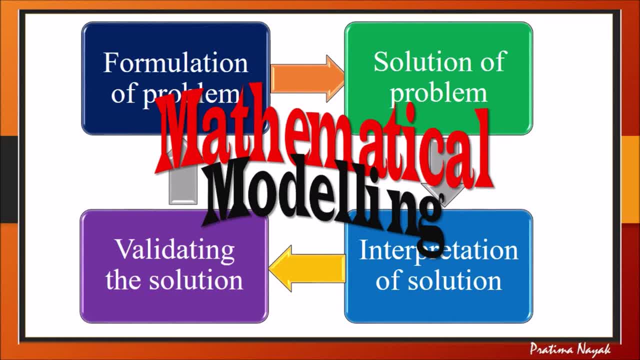 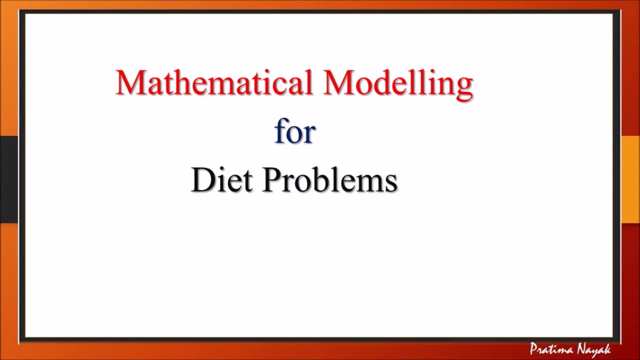 so today our topic is mathematical modeling in for diet problems. this is the project introduction. the process of constructing mathematical model is called mathematical modeling. a mathematical model is a mathematical relation that describes some real-life situation and has to tell. modeling helps us to solve the problems related to population explosion, spreading of an dynamic 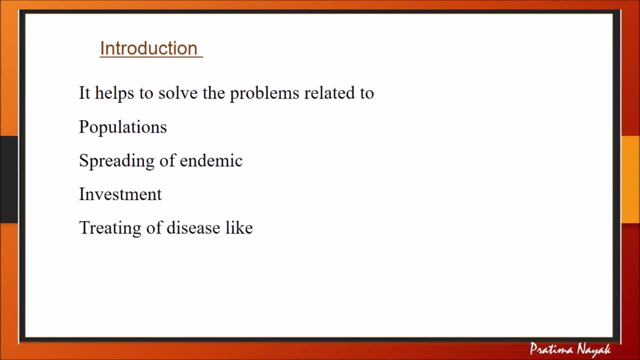 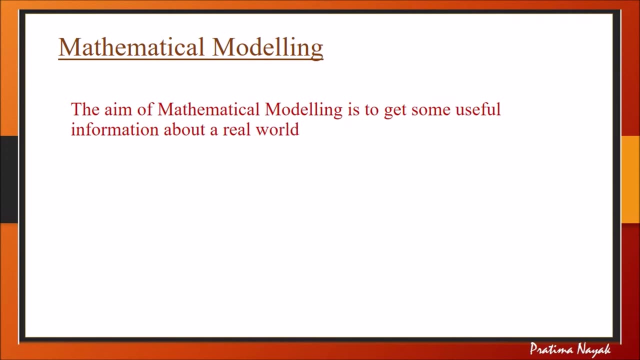 investment, treating of disease Call Mahatma, such as cancer and nutrition. The aim of mathematical modeling is to get some useful information about a real-world problem. by converting it into a mathematical problem, we solve the mathematical problem and interpret its solution in terms of the 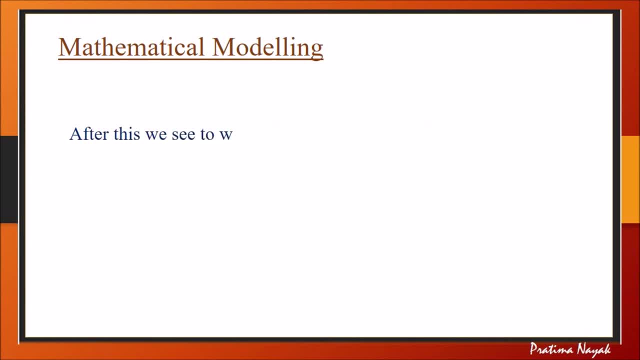 real world problem. after this, after finding the solution, we see to what extent the solution is valid in the context of real world problem. So let us discuss the real-world problem steps of a mathematical formulation of problem, finding the solution, interpreting the result and last is validation. Specific objective of modeling for 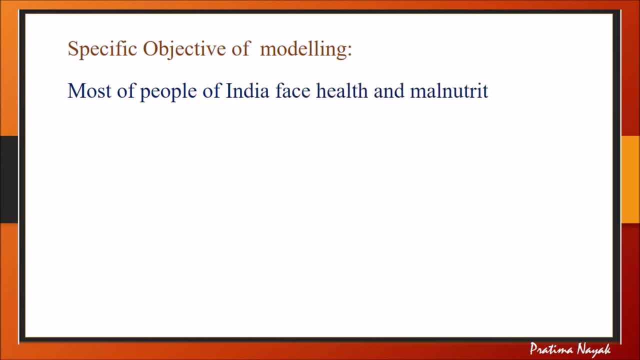 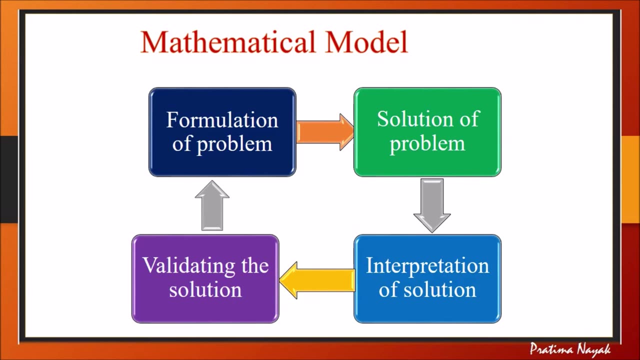 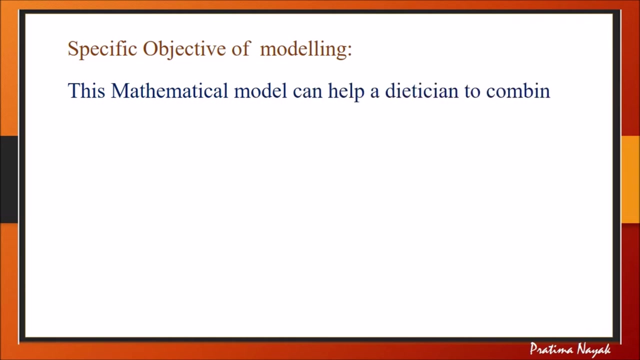 this particular case is. most of the people in India face health and malnutrition problem. some of them do not get proper nutrition due to lack of so a model is given here in the figure first. in this particular example we have taken a dietitian problem that this mathematical model can help a dietitian. 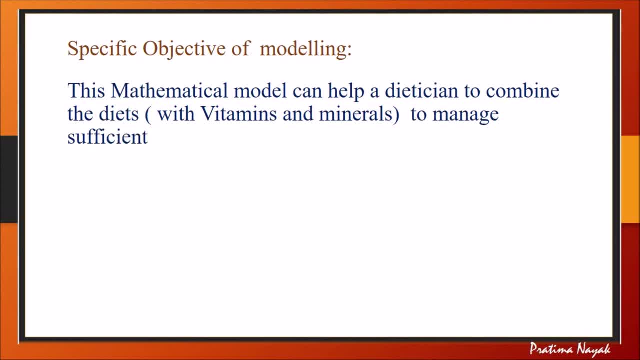 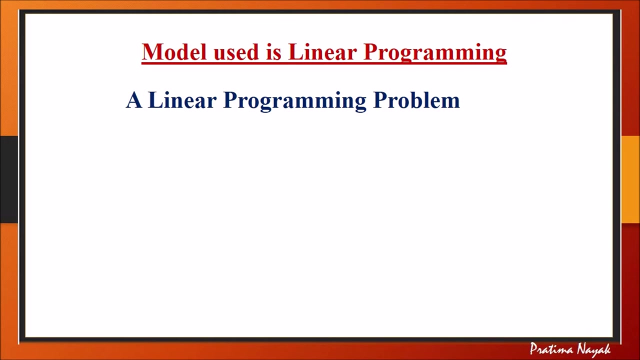 to combine the two problems, to combine the diets with vitamins and minerals, to manage the sufficient nutrients with a. so other important objective of this modeling is it will create an awareness that with minimum cost of the nutrition diet, various models are used in mathematical, as mathematical model to solve real-life problems. here we have: 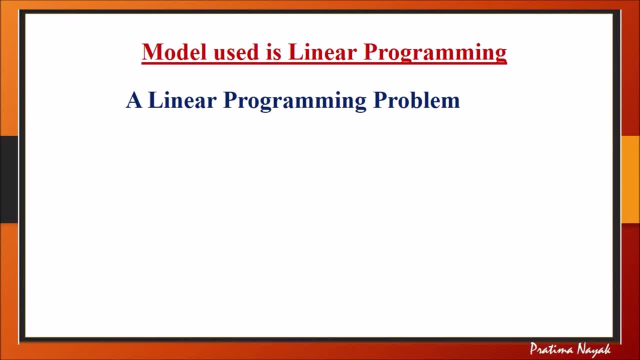 used linear programming or linear programming problem. now procedure step 1. step 1 is formulation of the problem. here we have formulated the problem. it is a diet problem. now, here there are some sub steps. one is stating the problem. now, here there are some sub steps. one is stating the problem. 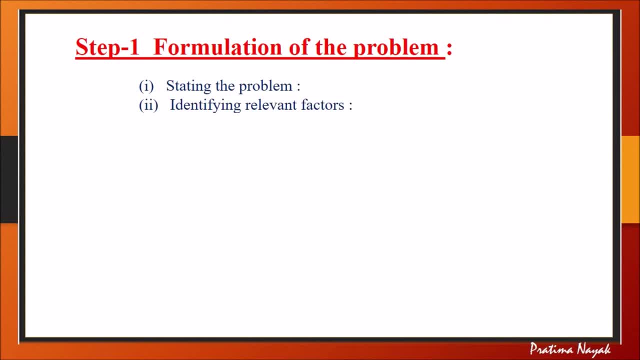 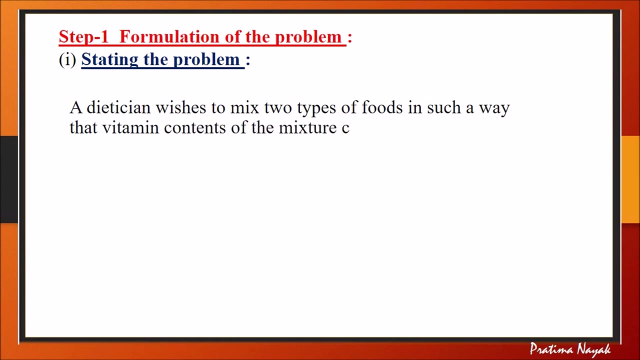 troubling is a diet is young. wishes to mix two type of foods in such away that ill go one by one, so stating no problem in that is young. wishes to mix two type of foods in such a way that vitamine contains of the mixture contain at least eight units of vitamin A in even. 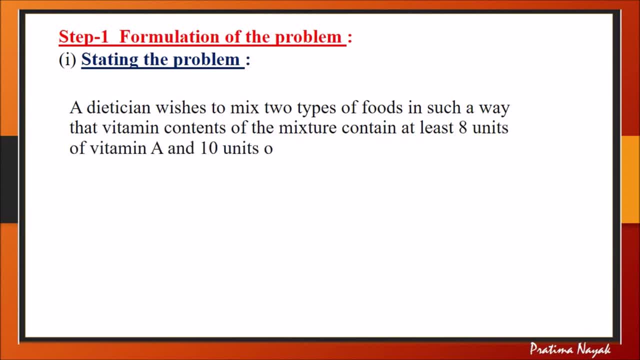 operation will result in嚴密 Ram Bediah madhya and 10 units of vitamin C. Food type 1 contains 2 units per kg of vitamin A and 1 unit per kg of vitamin C, Whereas food type 2 contains 1 unit per kg of vitamin A and 2 units per kg of vitamin C. 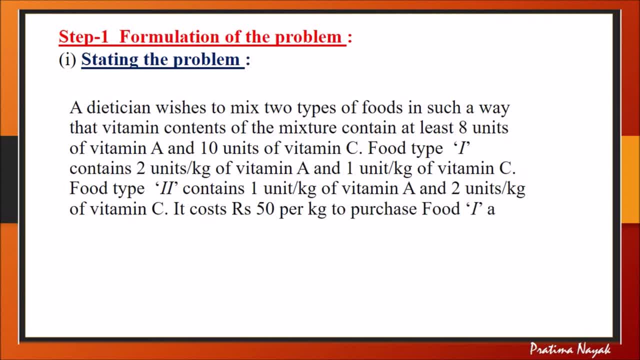 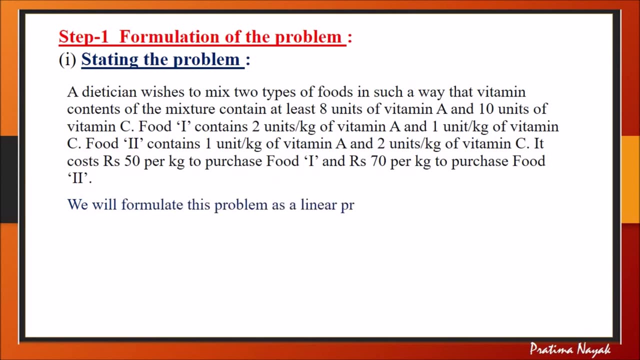 It costs Rs 50 per kg to purchase food type 1 and Rs 70 per kg to purchase food type 2.. We will formulate this problem as a linear programming problem, because we are applying this model here to minimize the cost of such mixture. 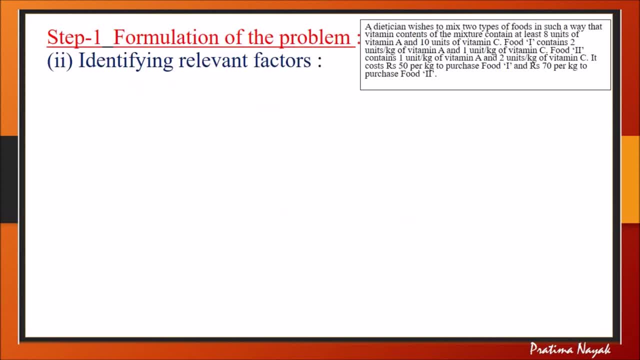 Identifying the relevant factors. Now we will go through the problem and we will find what are the relevant factors here to find the solution. First is amount of food type 1, and amount of food type 2 are not known. They are unknown here. 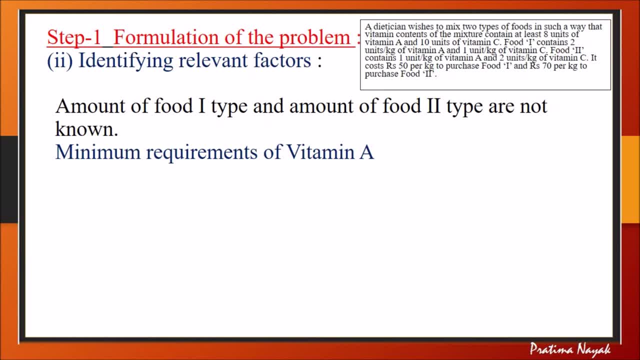 Minimum requirements of vitamin C. Vitamin A is given priority. Minimum requirement of vitamin C is also priority. Total cost is to be minimum. here This is the most important thing: to find that cost, which should be minimum. None of the amount is negative. These are the relevant factors for this problem. 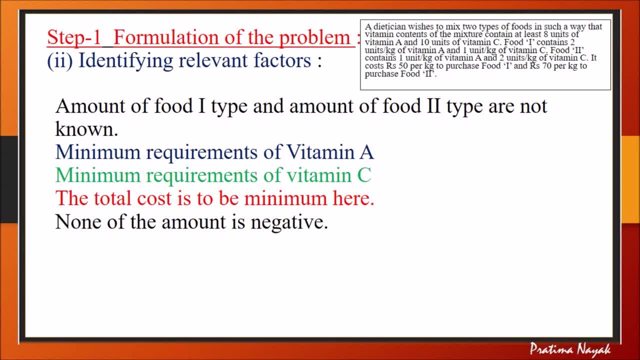 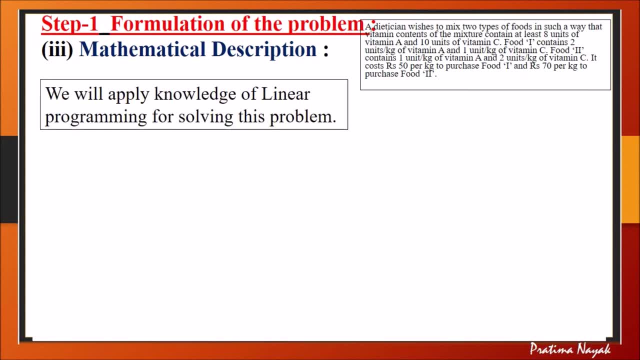 Now mathematical description of this problem. We will apply knowledge of linear programming for solving this problem. There are two unknown quantities. one is the amount of food type 1 and other is food type 2.. Let the mixture contain x kg of food type 2 and x kg of food type 3.. 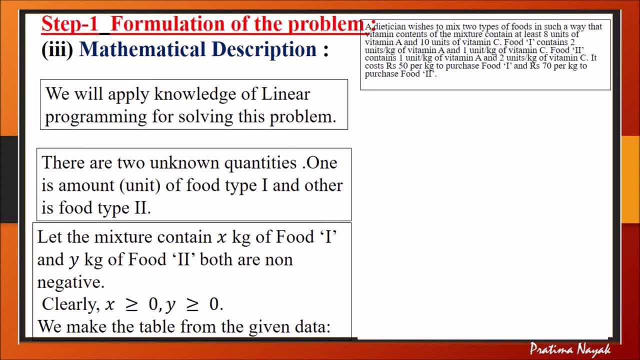 Let the mixture contain x kg of food type 2 and x kg of food type 3.. of food type 1 and Y kg of food type 2. both are non-negative. Clearly, X and Y. both are greater than equal to 0.. Now we will make a table of this given data. 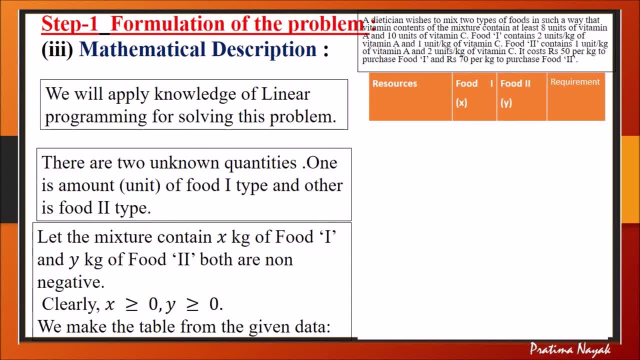 First is resources, food type 1, food type 2 and requirement. So vitamin A unit per kg and food type is X. it has 2 units of vitamin A, whereas food type 2 has 1 unit of vitamin A per kg and minimum requirement is 8 unit. 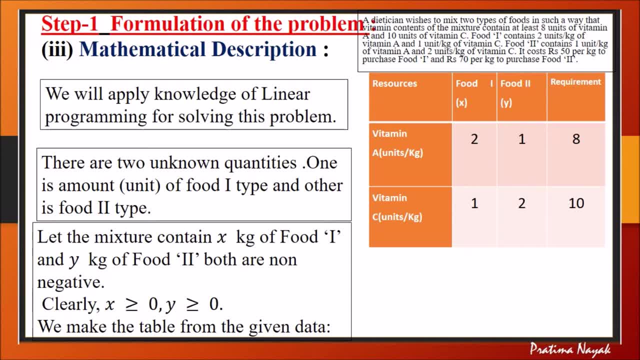 And vitamin C requirement is 0.. So vitamin A per kg and minimum requirement is 0.. For food type 1, it has 1 unit per kg and vitamin C in food type 2 is 2 unit per kg and its requirement is minimum 10 units. 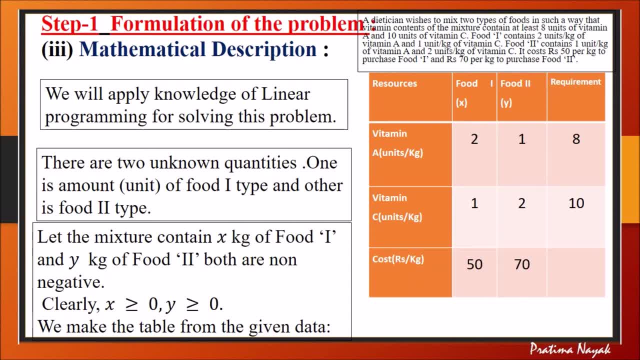 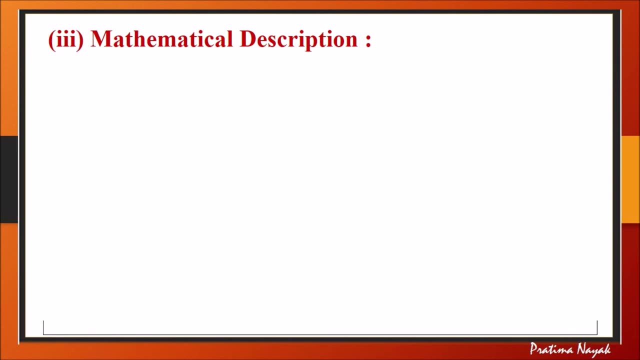 And if you will see the cost, food type 1 is Rs 50 per kg and type 2 is Rs 70 per kg and we have to find the minimum cost. So, mathematical description: Total cost will be taken as Z for per kg. 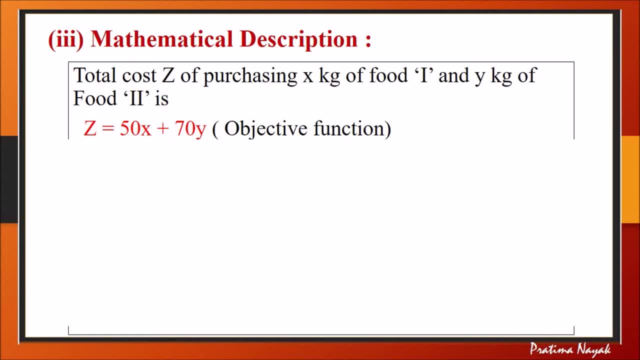 Purchasing X kg of food type 1 and Y kg of food type 2 is: Z is equal to 50X plus 70Y, because per kg of X type is 50 and per kg of Y type is equal to 70. Hence the mathematical formulation of the problem is: 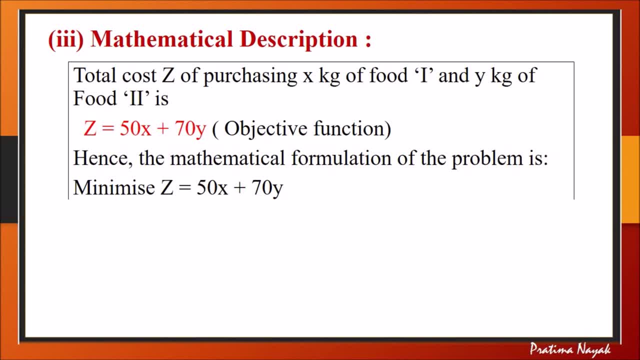 Minimize Z function is equal to 50X plus 70Y. We have to find out: Subject to the constraints, 2X plus Y is greater than or equal to 8, because minimum 8 should be there. Vitamin C X plus 2Y should be greater than or equal to 10.. 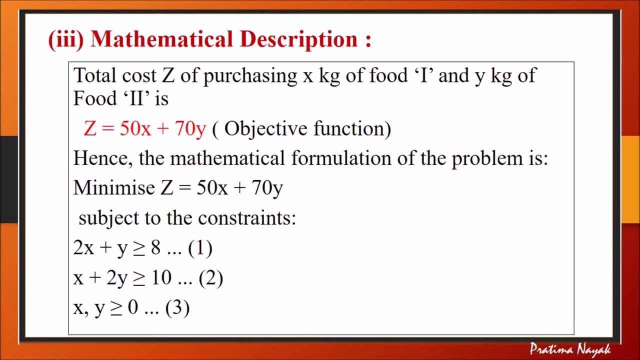 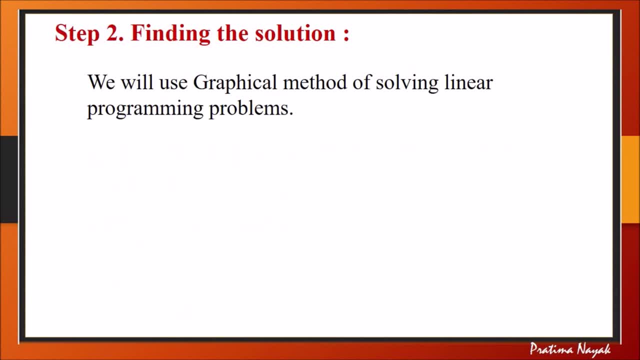 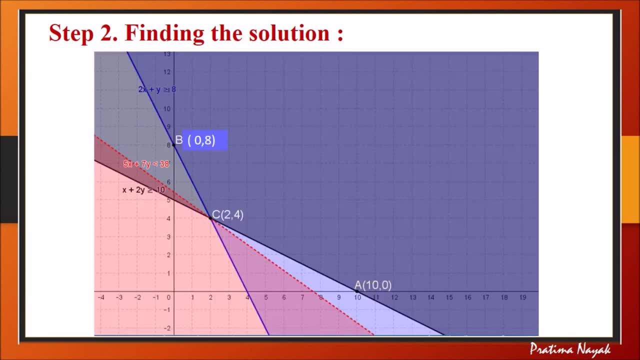 Both are non-negative. Next we will discuss Draw the graph of these constraints. We will use graphical method for solving linear programming problem. This is the graph. It is drawn with help of software GeoJabra. Here three equations are given as: 2X plus Y, greater than or equal to 8- blue line, and 5X plus X plus 7.. 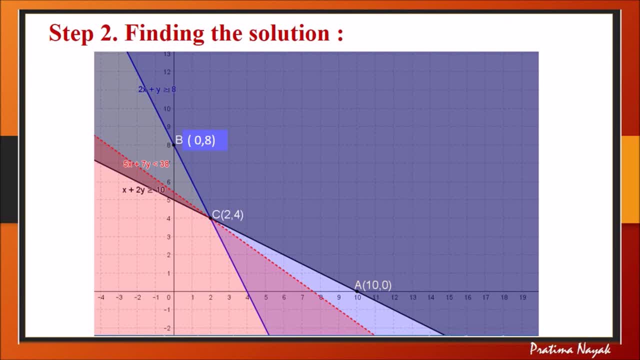 with help with cross color re- tray And delta: P plus X plus Nano, E plus T plus bitcoin Andatz向 y is equal to 10, that will be the black one, And in equation is drawn in this way: And x greater than zero, y greater than zero. 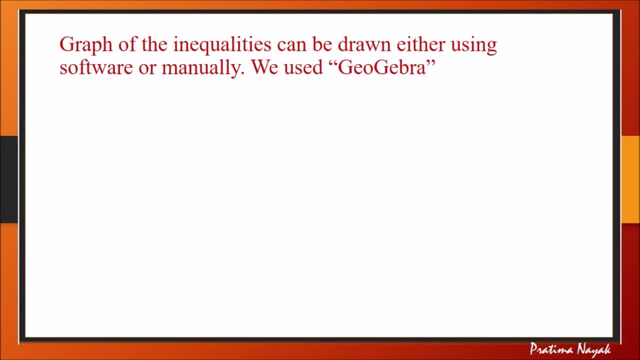 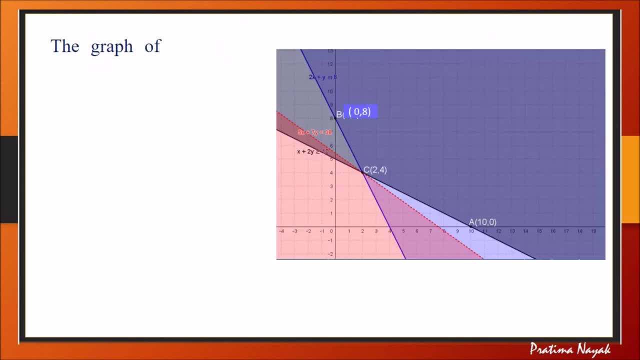 Certainly, it is the first quadrant. So, as I told, We have used GeoJabra. The graph of these systems consists of the point common to all half of the plane determined by the inequalities. The region, therefore, is called the feasible region for the problem. 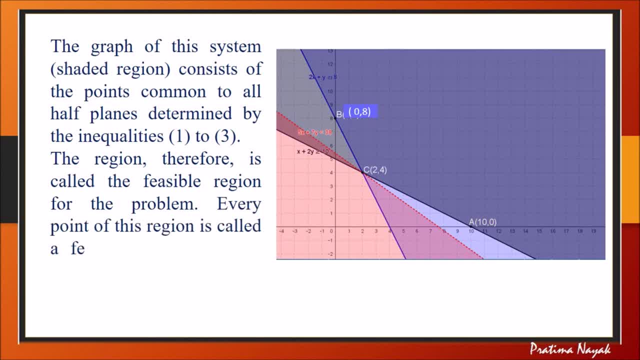 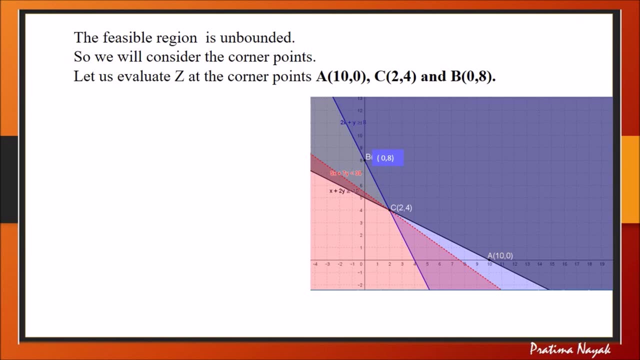 Every point of this region is called the feasible solution. The feasible solution is here unbounded, so we will consider the corner points. Let us evaluate the objective function z at each of the corner point. One is a 10,0 c. it has the coordinates 2,4. 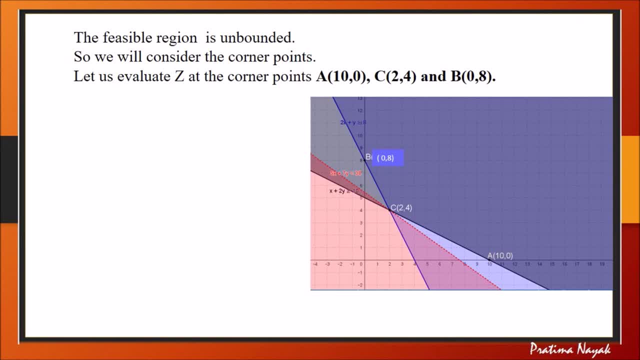 and b has the coordinates 0,8.. Now at b the value of this objective function is 560, because here x is 0,y is 8, and if we put in this equation 50 into 0 plus 70 into 8.. Next we will go. 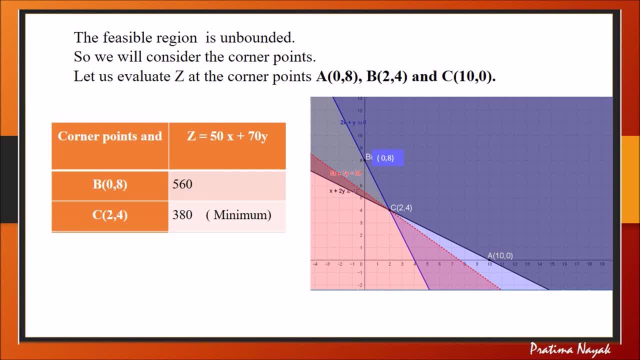 for point c, It will be x is 2 and y is 4. it gives minimum 380 and at a, if we will calculate, it will be: the value of this function is 500.. Now we have to find out which one is minimum. 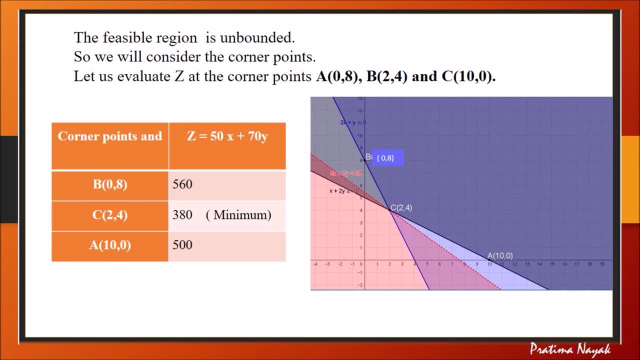 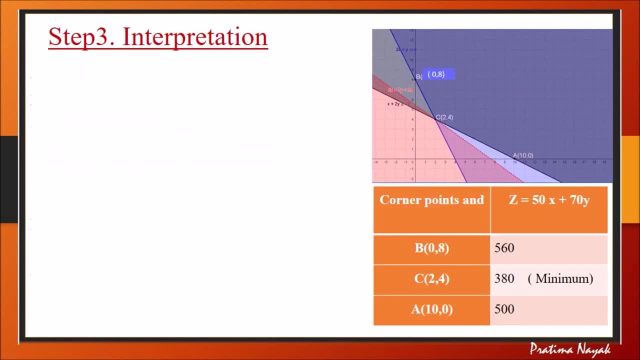 So minimum is at c, where x is 2 and y is 4.. So next is step 3, interpretation. From this table we will interpret which one will be the minimum cost. So we find the smallest value of z is at 380.. 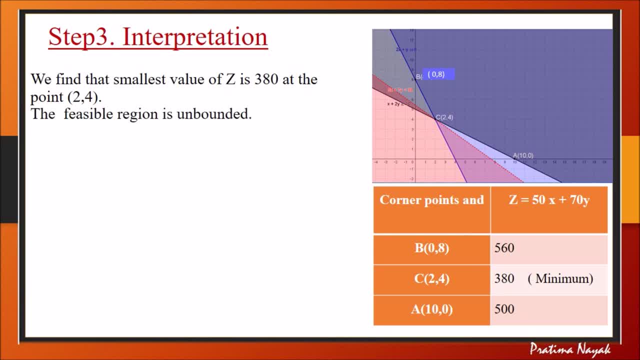 At the point 2,4.. The feasible region is unbounded. Therefore you have to draw a graph of inequality- 50x plus 70ye is less than 380- to check whether the resulting open half plane has any point common with the feasible region. 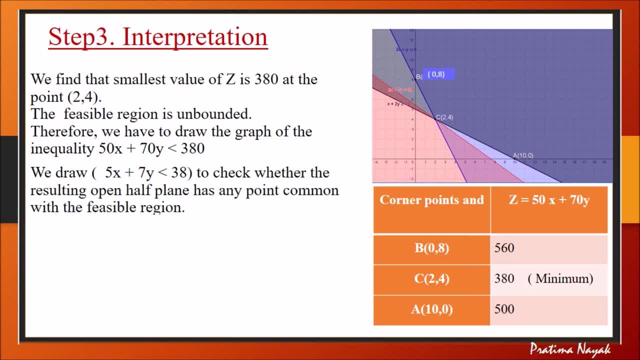 We draw 5x plus 7ye, less than 38, to check whether the resulting open half plane has any point common with the feasible region. From this figure we see that it has no point in common. This means that it has no point in common with the feasible region. 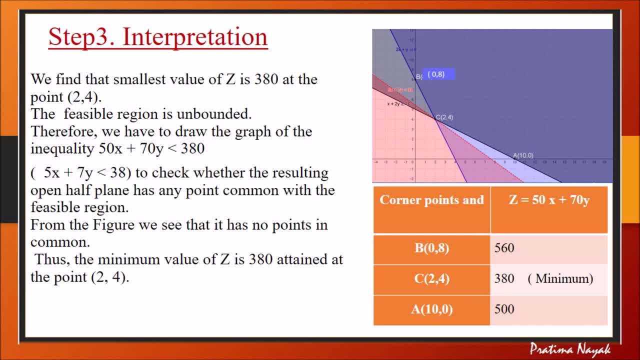 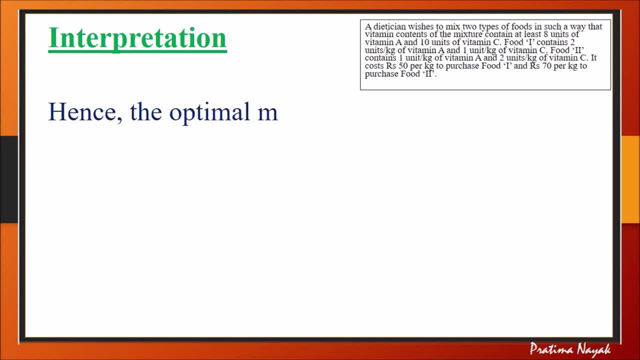 Thus minimum value of z is 380 attains at the point 2,4. So interpretation is hence: the optimal mixing strategy for the dietitian would be mix 2 kg of food type 1 and 4 kg of animal products and 4 kg of food type 2, and with this strategy the minimum cost of the mixer will be rupees 380.